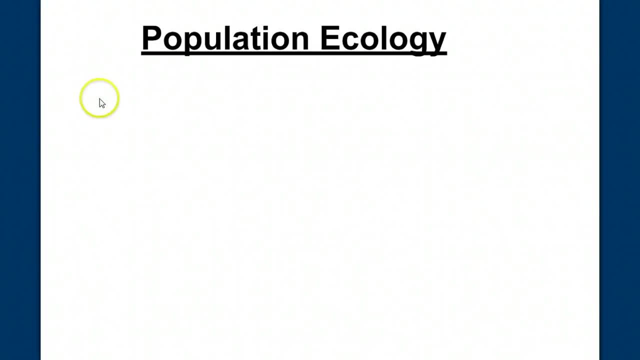 In this video we're going to look at population ecology. The first thing we need to do is look at the demographics of a population. Demographics include things like population size. The population size, the number of individuals that share a population's gene pool, will be determined and influenced by the intrinsic rate of growth of that population and also limiting factors. Another component of demographics is population density: the number of individuals in a given area of habitat. 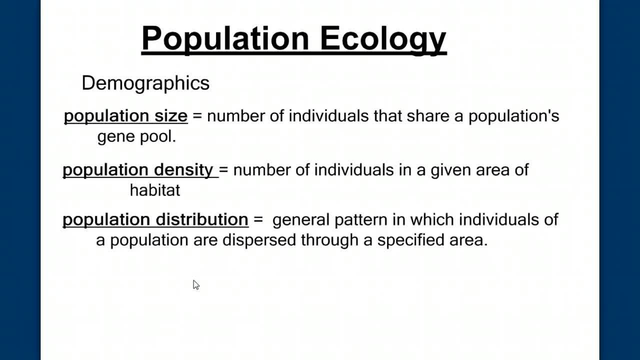 We'll also look at population distribution: What's the pattern in which the individuals of a population are spread out through the specified area? And finally, we'll look at age structure: How many individuals at each age level in the reproductive base, And how does this impact the future of the population? 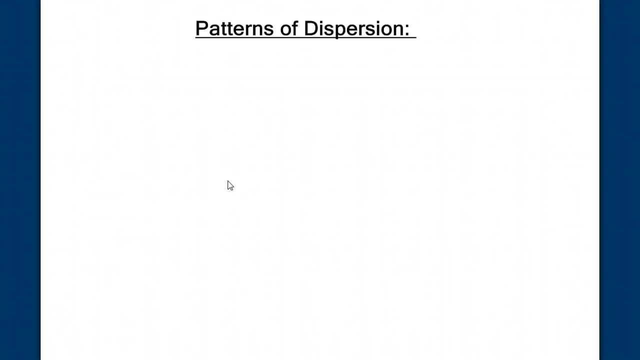 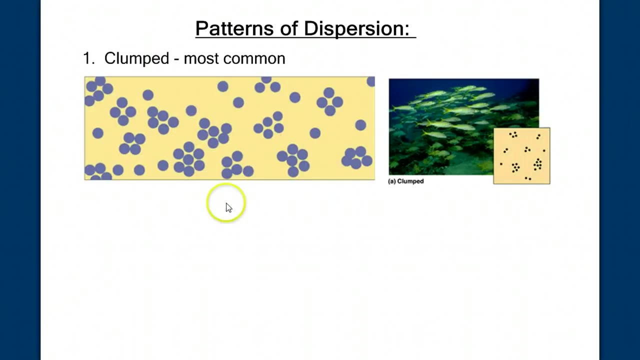 Let's start with patterns of dispersion. The most common pattern of dispersion is called clumped And it looks like this: Organisms are spread out throughout the habitat, but they're not spread out in a homogeneous manner. They clump together in these clusters. 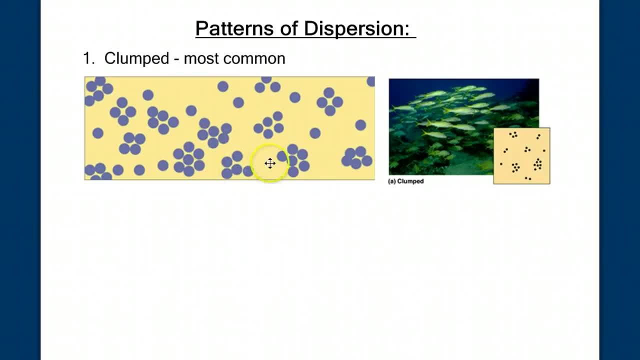 The question is twofold: Why are they clumped in these clusters And why is this the most common pattern? Take a minute to consider these questions. Stop the video and write down a few reasons why you think that clumped would be the most common pattern of dispersion of organisms within an environment and what's the cause of this clumping. 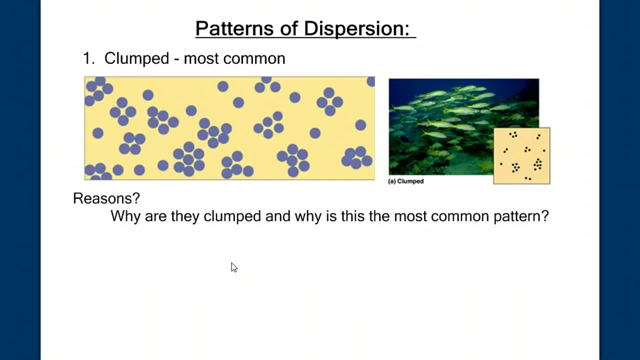 What ideas did you come up with? What is it that they'd be clumping around? What is it that they'd need to stay near? Well, probably, resources like food and water. Species are adapted to a limited set of environmental and ecological conditions, And those conditions are patchy. within a habitat, They're heterogeneously distributed. 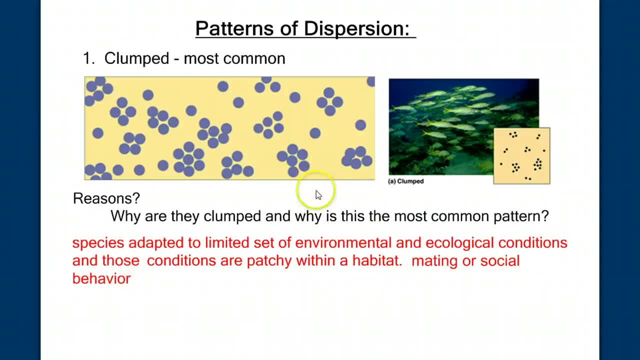 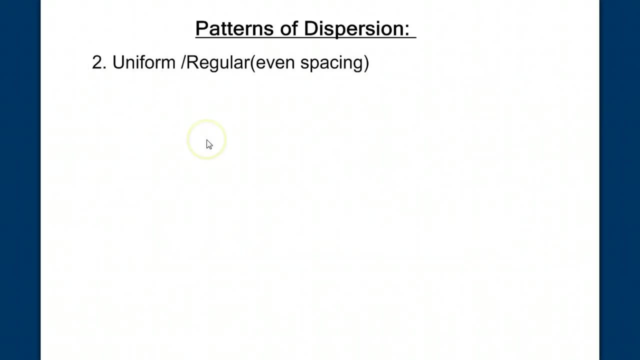 So we would expect that the organisms would also be heterogeneously distributed around those populations. We'd expect that they'd have pockets of resources And also from mating and social behaviors it makes sense for organisms to clump together. Our next pattern of dispersion is uniform or regular, where we're seeing even spacing of organisms throughout the environment. 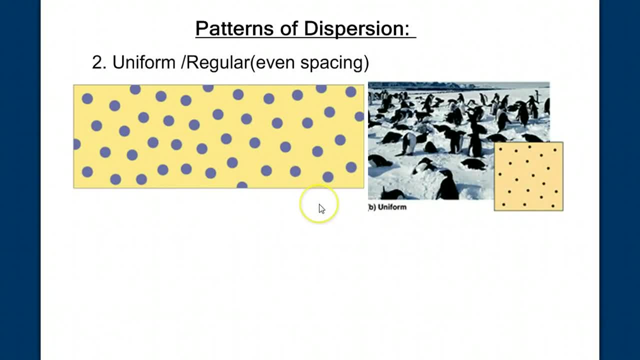 Under what conditions would you see organisms spread out like this, with this kind of even spacing between them? Stop the video and write down why you think this could happen. Why, when we look from above, do these penguins all have a very specific amount of space around? 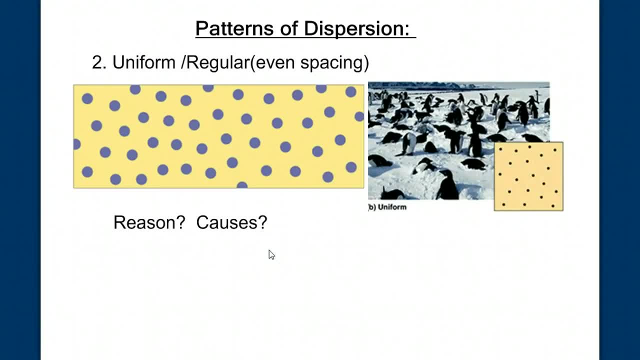 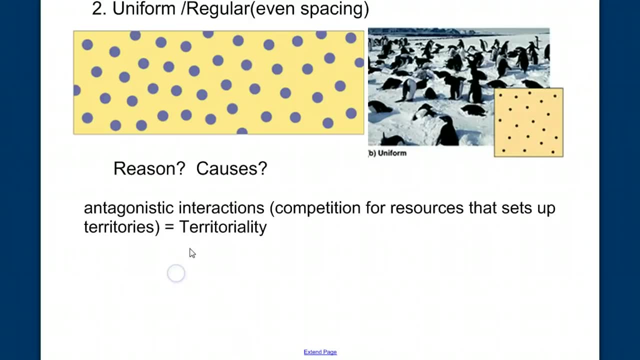 them, and they don't tend to encroach on each other's space. What ideas did you come up with? The answer has to do with competition. Antagonistic interactions are competition for resources that sets up territories. This territoriality allows them to avoid conflict by carving out their own space. 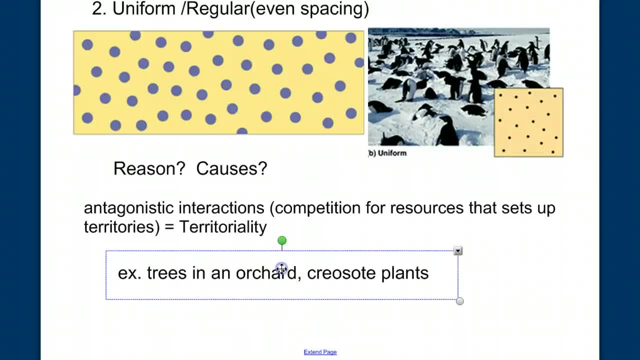 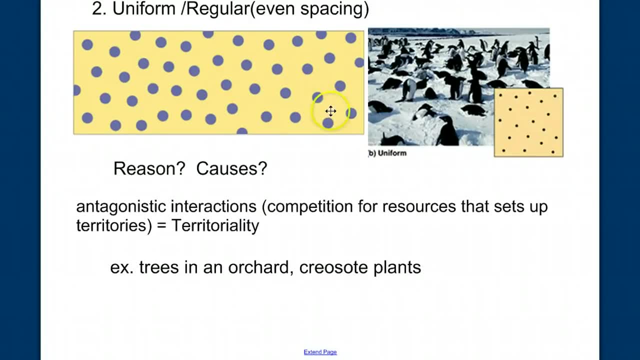 Some examples would be trees in an orchard, or these penguins, or the creosote plant, which does something very interesting. If you flew over an area where there are a lot of creosote plants, it might look like this picture here: 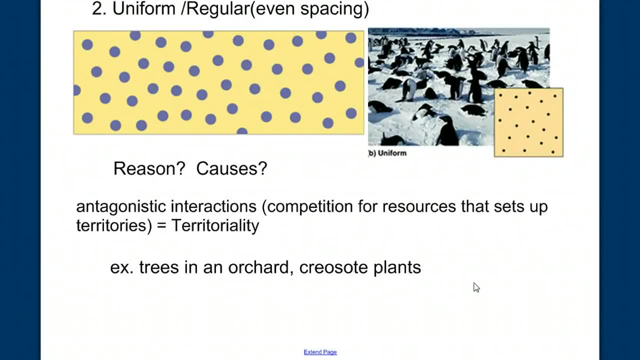 It's almost as if the other creosote plants know not to encroach on each other's area. What happens is the creosote plants secrete an oil that, when it drops to the ground, prevents any seeds in that area from germinating, thus carving out space for itself. 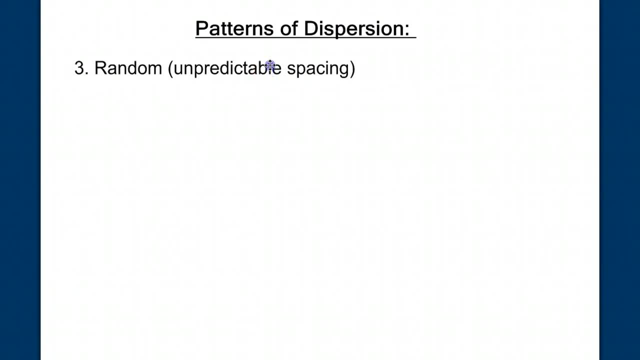 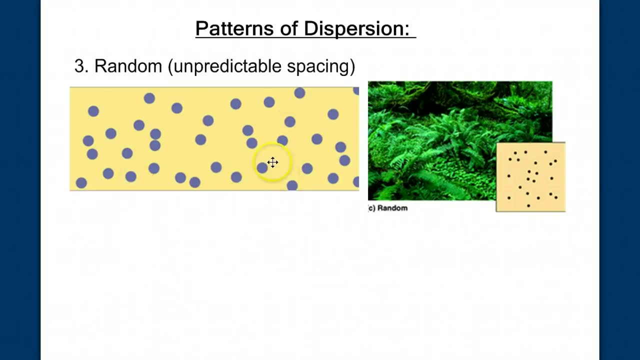 Our third and final pattern of dispersion is random, where we see an under-predictable spacing. Again, the question is why, Under what conditions, would we see this pattern where there seems to be no reason to stay away or no reason to clump? 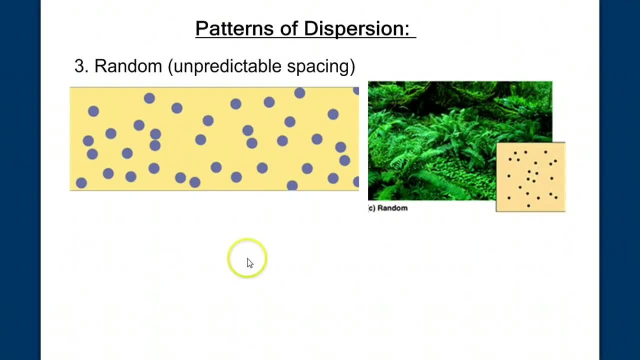 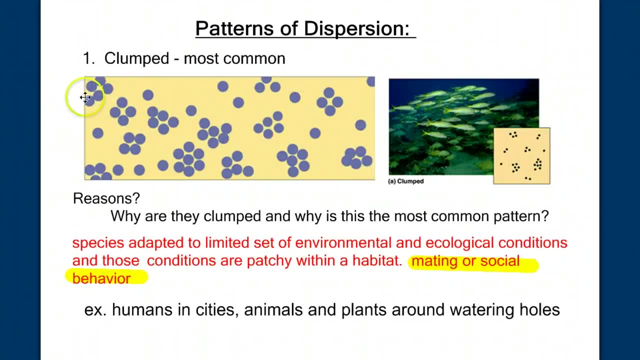 Pause the video and think if you can come up with the conditions under which we'd get this type of pattern of dispersion, If clumped is the most common and organisms tend to clump around resources like human beings would in a city, or animals and plants around a watering hole, and uniform and regular 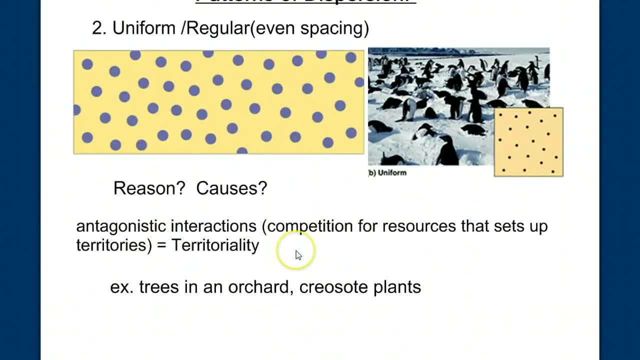 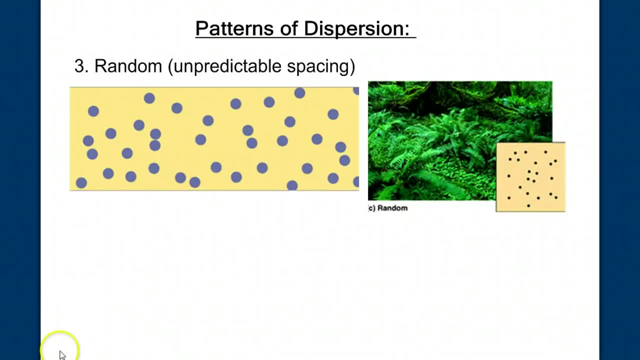 is due to large amounts of competition, creating situations of territoriality. why would we get a situation where it's random, What conditions would be present or lacking? Well, we'd have a fairly uniform distribution of resources, rather than an uneven distribution. 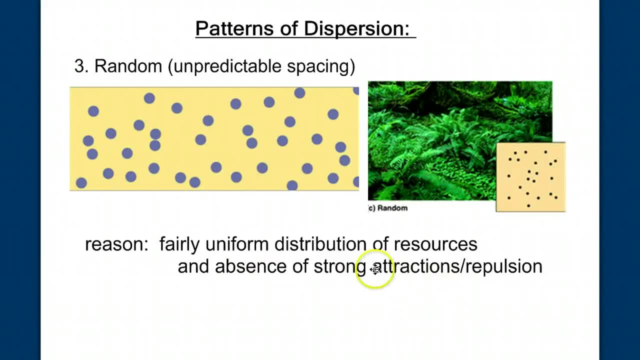 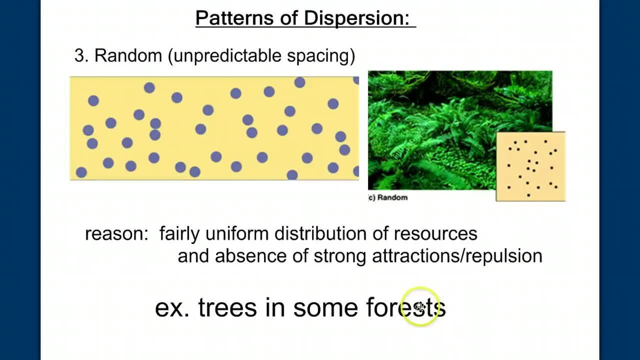 and it's the absence of strong attractions or repulsions that would lead to this random spacing. An example would be Trees in certain forests or these plants here in this picture that have access to the resources but have no reason to either attract or repel each other. 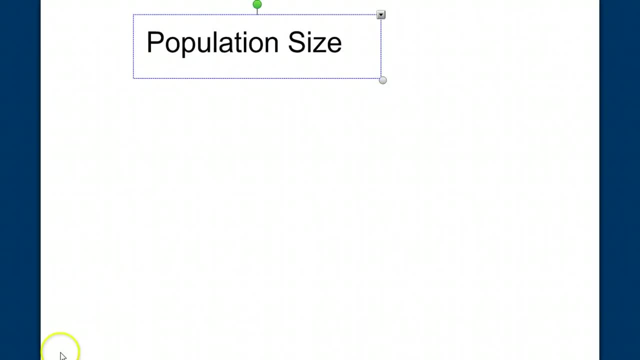 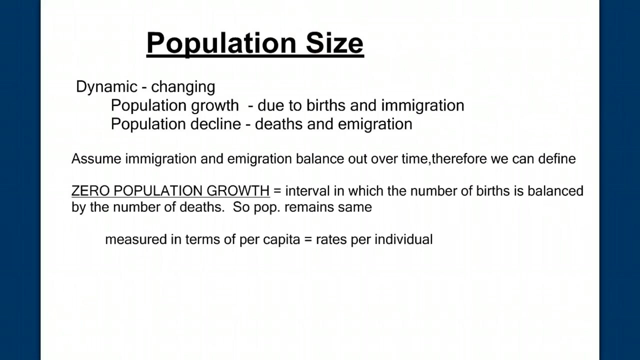 Let's move on to population size. Population size is dynamic. It's always changing. It grows due to births and immigration, or individuals moving in, and it declines due to deaths and emigration individuals moving out. If we assume that emigration and emigration are the same, then we'd have a situation 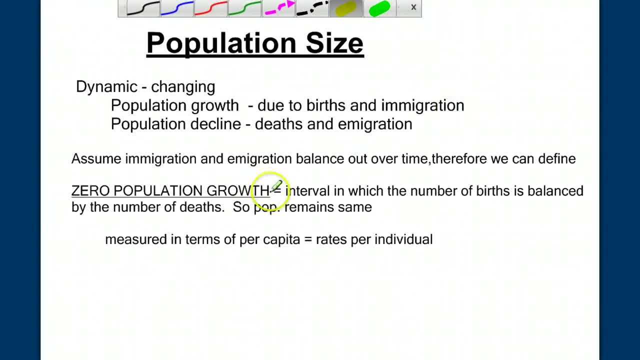 where the number of deaths and emigration will balance each other out over time. We can define zero population growth as the interval in which the number of births is balanced by the number of deaths, so that the population remains the same. We usually measure this in terms of per capita, in rates per individual. 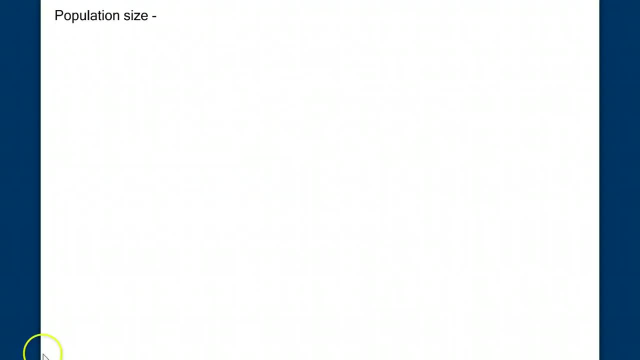 Let's work through an example. If we had, let's say, a population of 2,000 mice and in one month they produce 1,000 offspring, what would be the birth rate for this population? Let's look at an example. 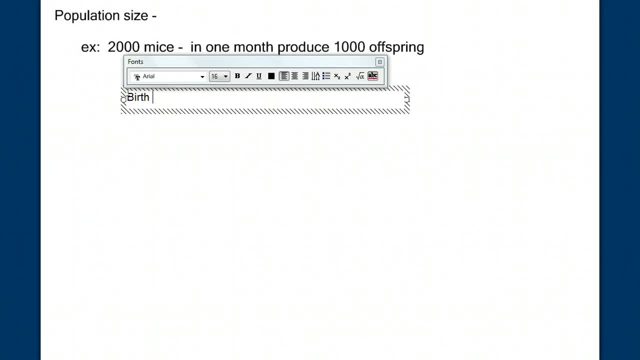 If we had, let's say, a population of 2,000 mice and in one month they produce 1,000 offspring, what would be the birth rate for this population? Well, the birth rate would equal the 1,000 produced divided by the 2,000 of the base. 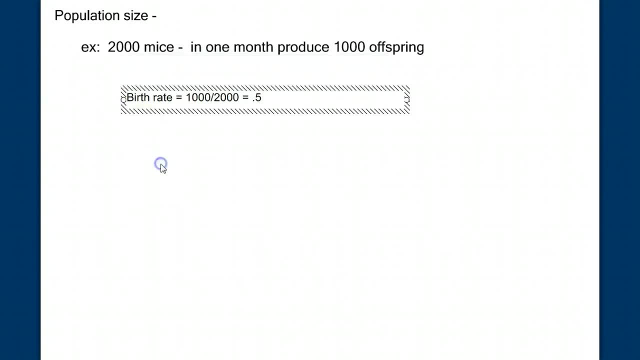 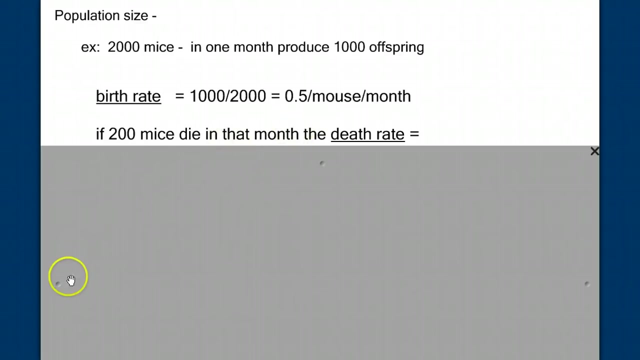 population would equal .5. That's in units of per mouse per month. If, during that same period, 200 mice die, what would be the death rate for this population? Stop the video and enjoy. If 200 mice die in that month, then the death rate would equal the 200 divided by the base. 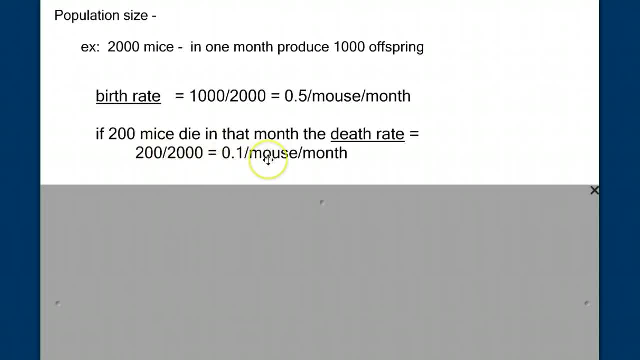 population of 2,000, which equals .1 per mouse per month. Now, then, to calculate the growth rate of this population, we need to take the number of births, or the birth rate minus the death rate, to give us our net overall rate of growth. 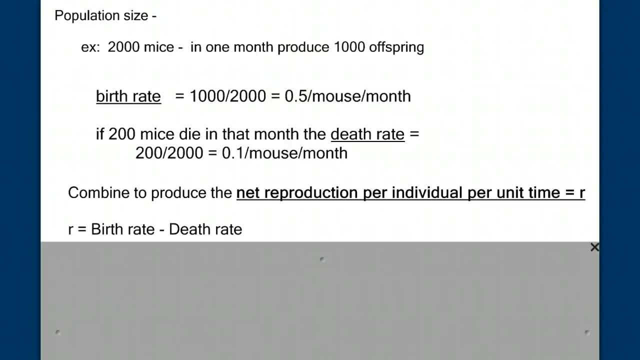 per unit time The birth rate minus the death rate, And we designate that with the letter r for rate. For our example, the rate or r is 0.5 minus 0.1.. So our overall rate of growth or net reproductive rate, 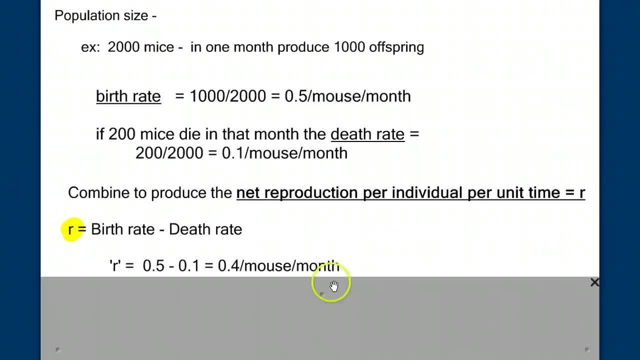 is 0.4 per mouse per month. Now I don't really know if mice populations grow at this rate. I made this example up as I go, But let's see what this means as we grow from one month to the next. 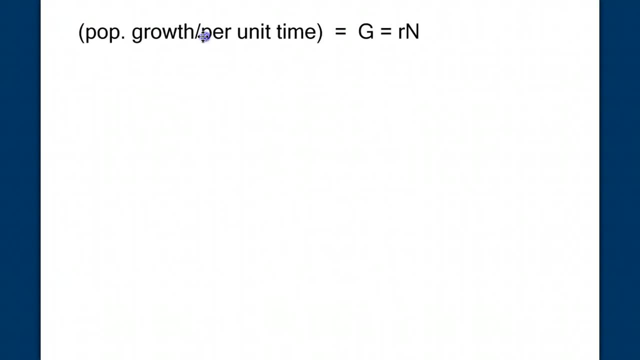 So this is the formula that we're going to use: The population growth per unit time, or the growth g, is going to equal r, which is our intrinsic rate of growth, which we just calculated times n, And n is our base population. 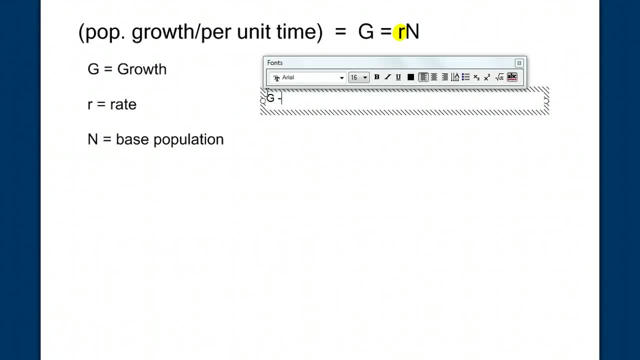 So for us we're going to have g in our example equals r, which is 0.4, times the population, which was 2,000. So that in one month's time we'd have a growth rate of 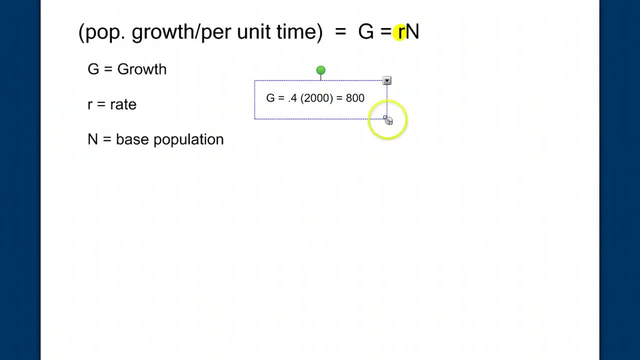 or we'd add up. We'd add 800 individuals to our population. So what's our population at now? We take this 800, we added net rate of growth, or net growth of individuals. We add it to our base population of 2,000. 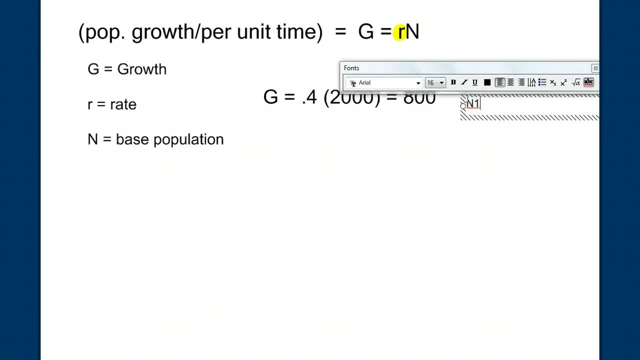 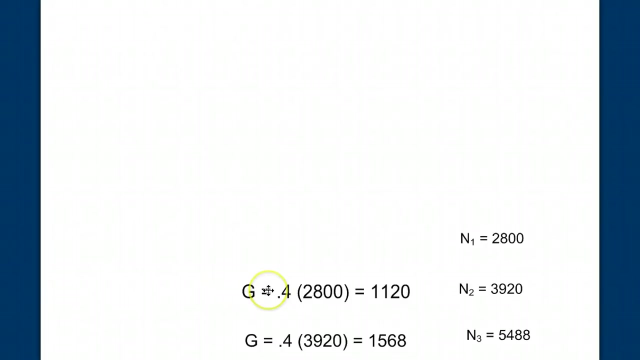 So our population at one month, or our n1, equals 2,800.. And the opposite is our base population, which is 1,500, which is 1,000.. So our family, as a result of this, is now 1,500. 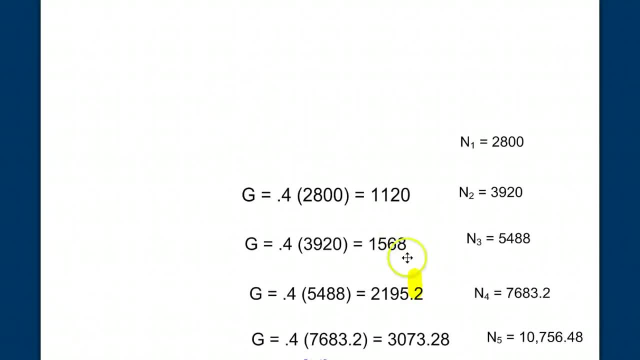 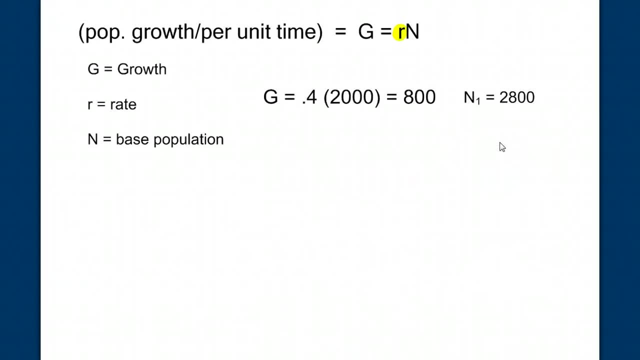 So we're going to add 2,000, plus 4,000, into the population, And then our net growth. So we're going to add 2,000, plus 3,000.. And then the increase of course. 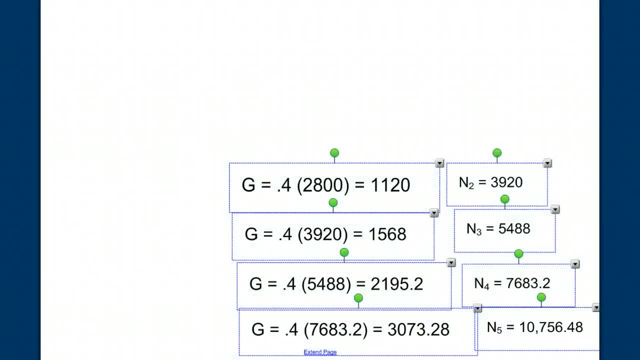 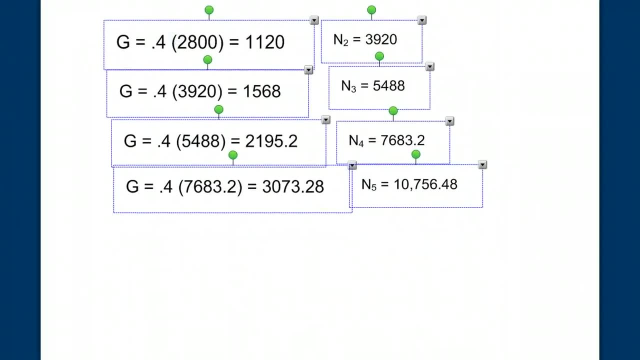 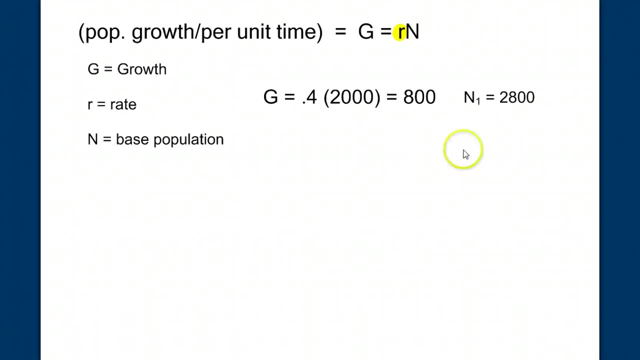 is going to be just 1,500, plus 1,000. And so the breaking down: we're going to add 1,000, plus 1,000. And we're going to add 1,000.. Now, what's going to happen the next month? 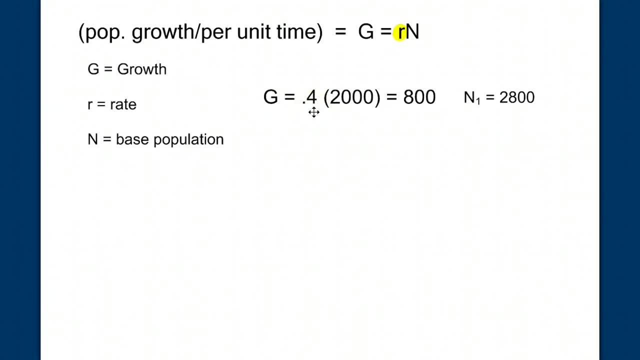 The next month our R, our rate of growth, doesn't change, but our N does change. We have now 2800 to grow from. So in month number two we have our 2800 person population, or mouse population, and we add another 1120 during the second month, which brings our population to 3920. 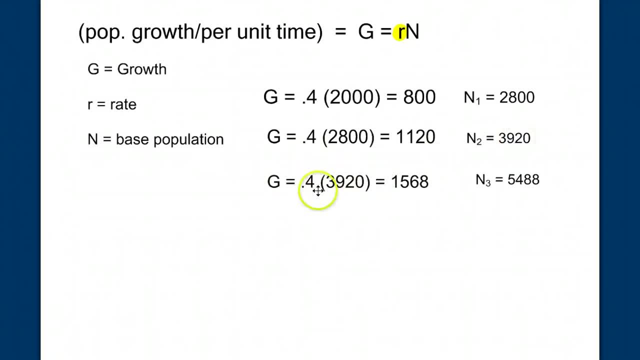 Let's look forward to the next month. The next month we multiply our rate of growth times, our new population size- 3920, and this month we add 1568,, bringing our population to 5488.. Now, what can you see happening? 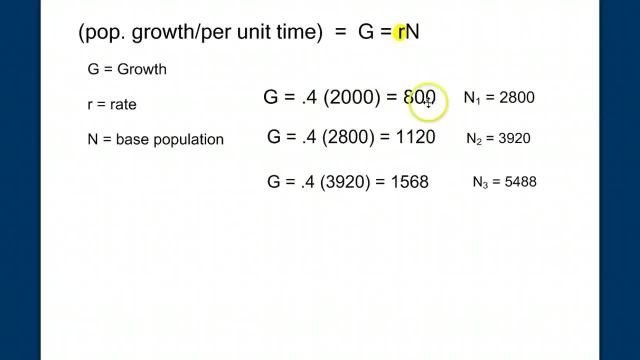 Each month, our rate of growth is the same, but our amount of growth, the number of individuals we're adding, is increasing Because our base population is increasing. Let's continue. We see that the next month we have an addition of 2195.2,. well, we can't have .2 of a mouse. 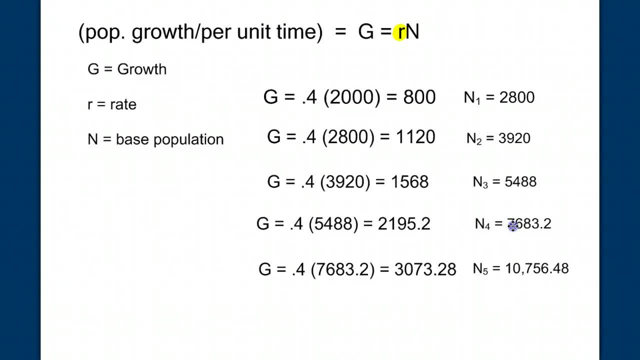 but that's what the math works out to be, which brings our population up to over 7600.. And the next month we multiply our rate of growth, times that number, and we add 3000 the next month. What we need to do is put this onto a graph. 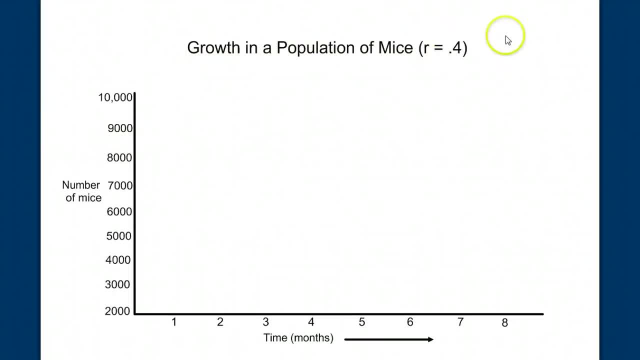 Here's what our graph would look like: The growth in a population of mice with an R of- Remember- R is birth rate minus death rate And we have our time in months down at the bottom and our number of mice on the side, starting with our original population of 2000.. 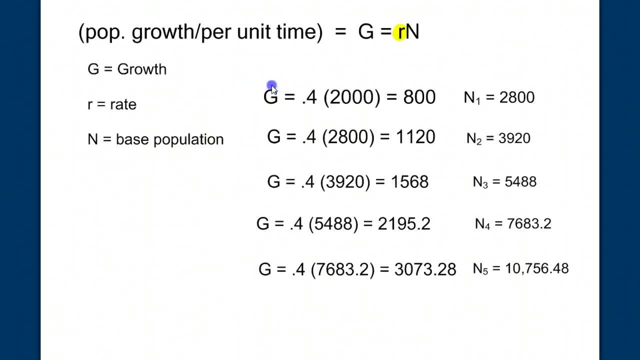 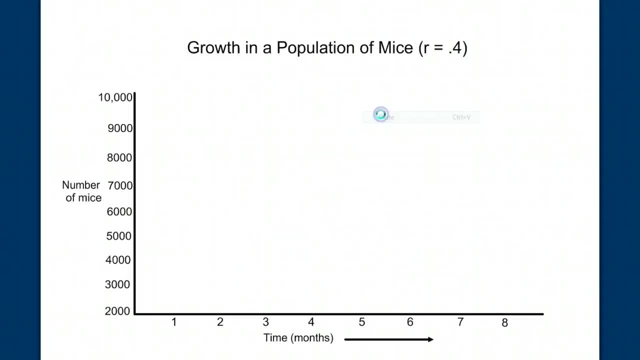 Let's bring our data over from the other page. Let's grab this, copy and paste that here for a moment. we'll make it smaller. give me one second. Okay, I made that smaller. now Let's pick a mouse. 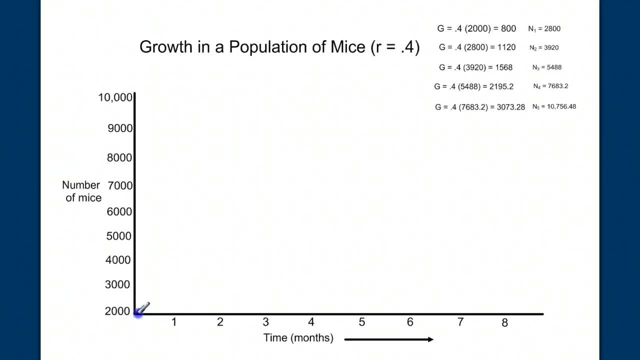 We have a pin and our original population is 2000.. And at one month we are at 2800, so right about there that might be a little high. And at two months we're at 3920, so we're nearing to 4000. 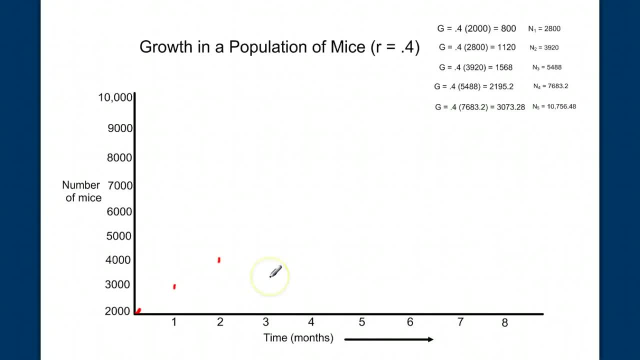 And at three months we are at 5488, so right about there. And then at four months we're at 7000.. Okay, At five months we are at 683, so I'll put a mark there. And at five months we are at over 10,000.. 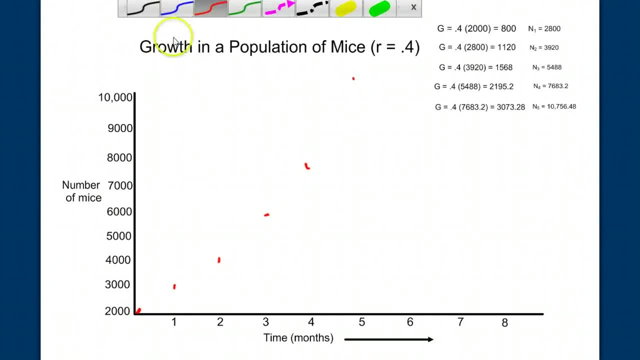 So let's see what the shape of that line looks like. Hopefully you can see that this line is- I'll grab a pin here- is the slope is increasing and eventually it will continue to increase and it can get steeper. 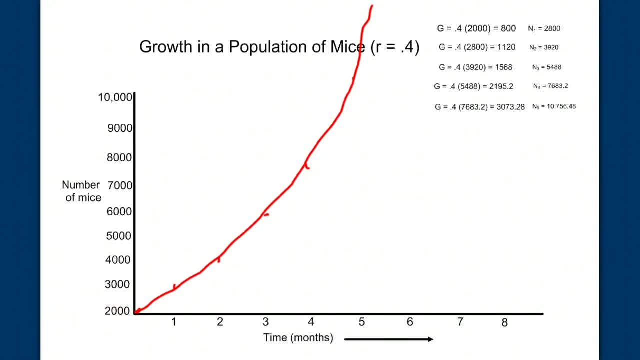 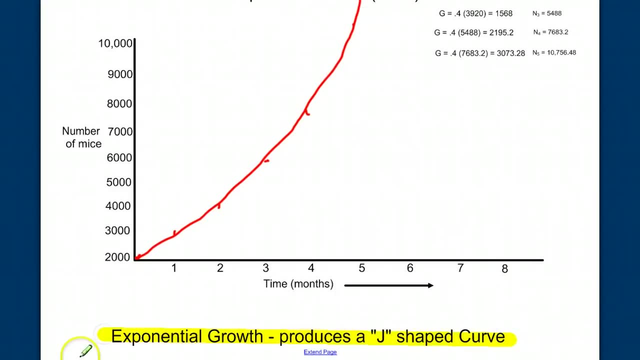 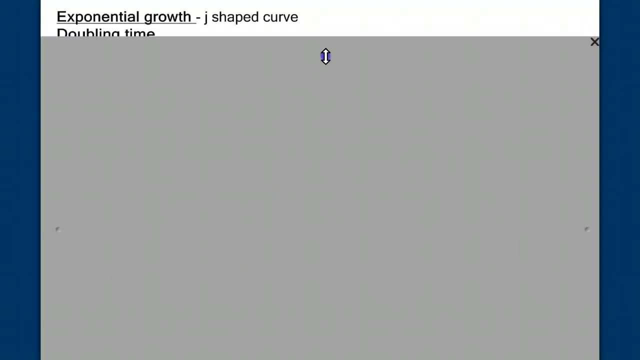 And we call this a slope, And we call this an exponential growth curve, and it gives us a J-shaped curve. Now this is what will happen to populations under ideal conditions, with nothing slowing down the rate of growth. We would say that this population is growing at its biotic potential, the maximum rate. 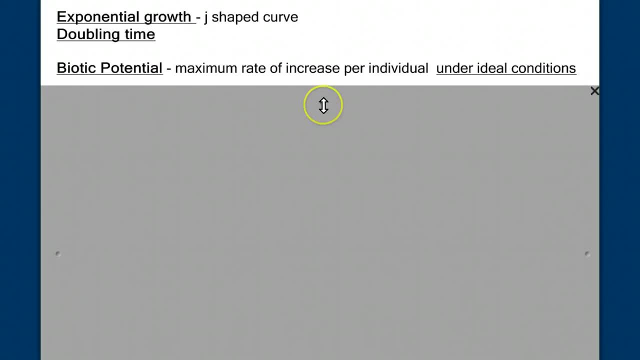 of increase per individual under ideal conditions, But we most likely don't have ideal conditions, and so the actual rate of growth depends on factors such as the age at which we're growing. Okay, So what we're going to do is we're going to look at how often we start reproducing. 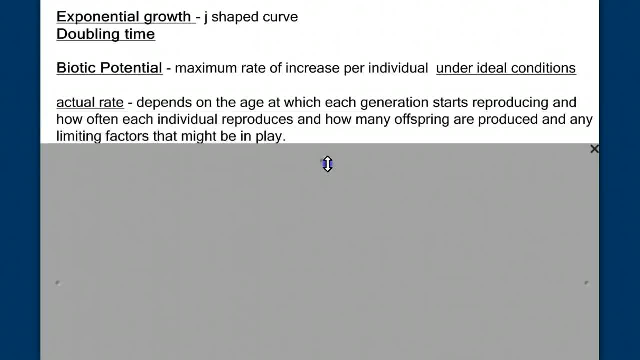 and how often each individual reproduces and how many offspring are produced, and the limiting factors that might be in play. Let's talk about these limiting factors and what they mean. Limiting factors are any essential resource that is in short supply and is a limiting. 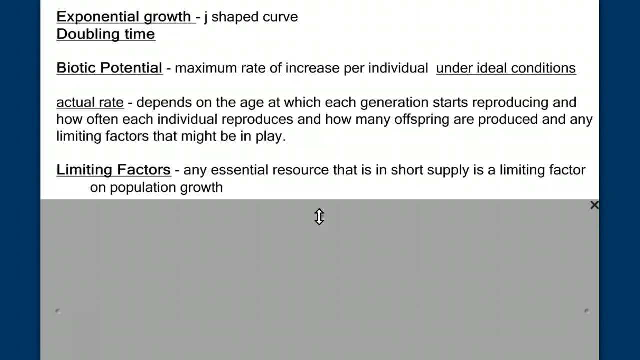 factor on the population growth. Stop the video now and write down all the things that could limit a population's growth. What types of growth? What types of things did you come up with? Probably food, maybe minerals, refuge from predators, places to hide space, just physical. 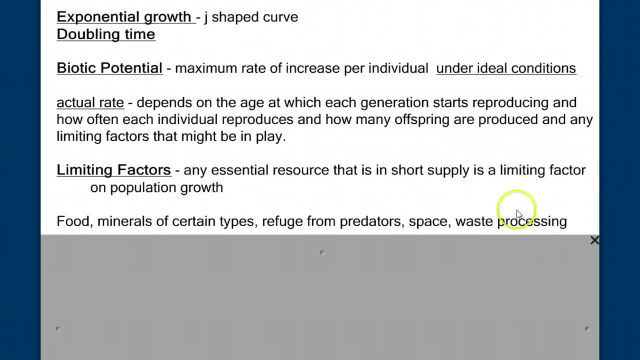 space and waste processing. You may be able to have a lot of individuals, but those individuals produce waste that we need to filter out of our environment. All those factors can limit how much a population can grow, and there is a theoretical maximum number of individuals that a population can sustain. 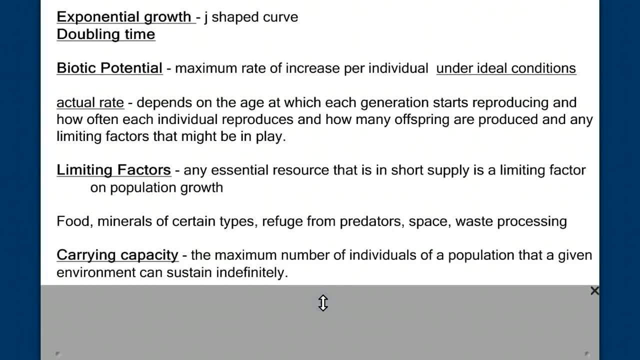 We call that concept the carrying capacity The maximum number of individuals of a population that a given environment can sustain indefinitely. We need to consider how that impacts our mathematical model, and so we're going to give it the letter K. K stands for carrying capacity, and we'll add that into our mathematical model. 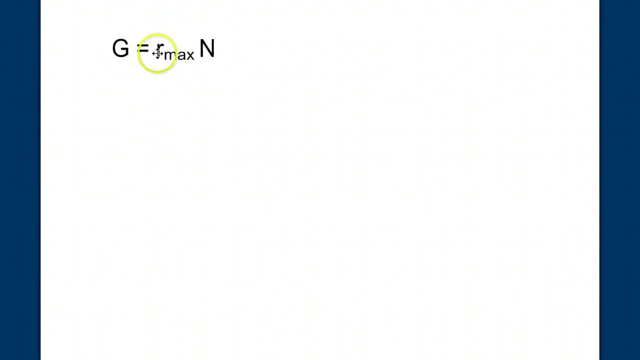 We'll start with the formula we had before. Growth equals the rate times the population size. We have the RMAP. That's the maximum rate of growth. We add to that the concept of carrying capacity, some number. that's the maximum that a population 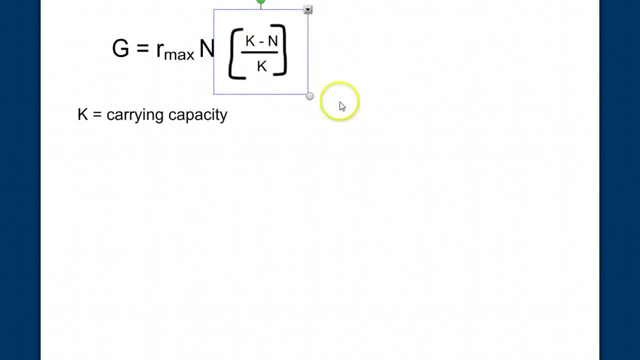 can sustain. and we create this factor, The carrying capacity minus the number of individuals divided by the carrying capacity, a factor of how close we are to that number, that carrying capacity number. We add that into this mathematical formula and let's look at what happens. 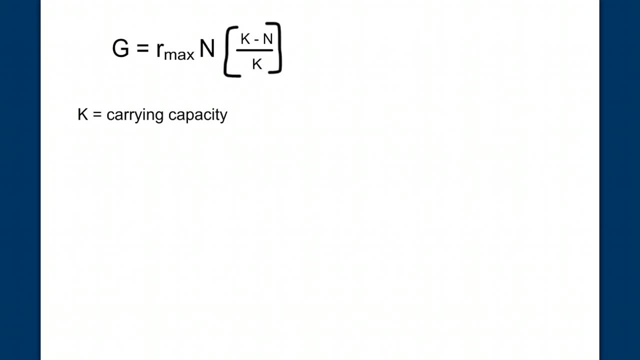 If N is relatively small compared to K, then this number, if N's very small, then subtracting N from K isn't going to change this fraction very much And this fraction will be near 1.. And if this fraction is near 1, then the population will be growing near its max rate. 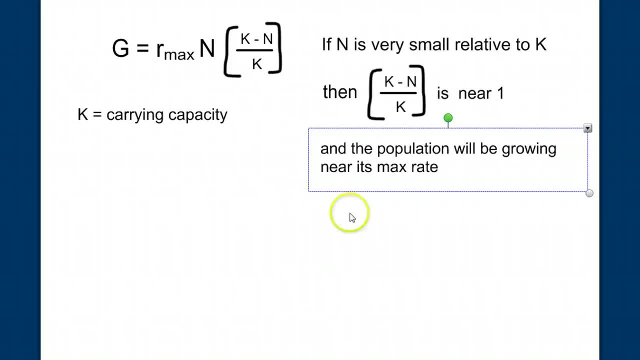 Take a second to digest that If N's small relative to K, then we're going to have to subtract the N from K. Why does that happen? Can we go back to that example? Why can we subtract the N from K? Why can we subtract the N from K? 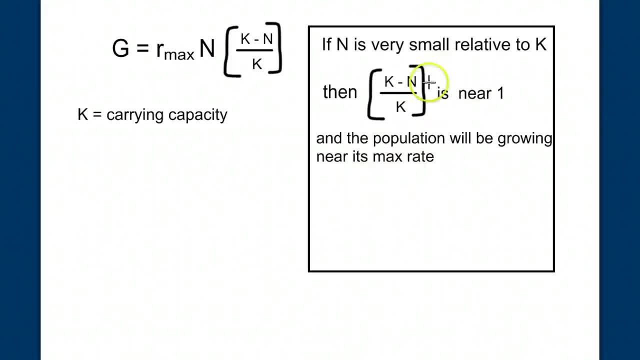 Okay, Okay, Okay. Okay, then this factor is nearing 1,, or close to 1,, and the population is going to grow near its max rate. But more interesting is to see what happens as n approaches k. As n approaches k, 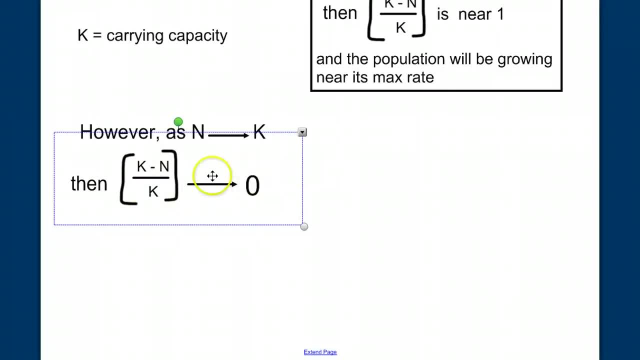 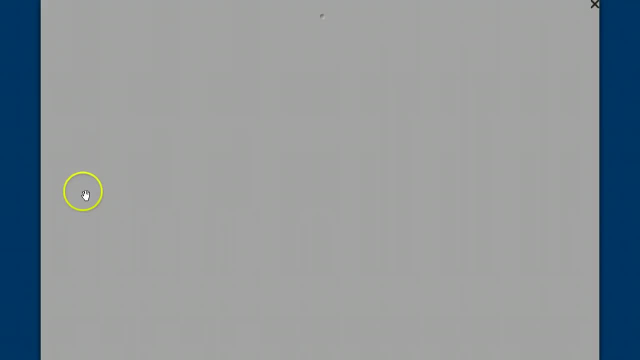 then this factor, k minus n, divided by k, approaches 0.. And therefore g approaches 0, and therefore the population growth will near 0.. We need to look at it graphically. When a population starts out growing, it'll grow small at first. 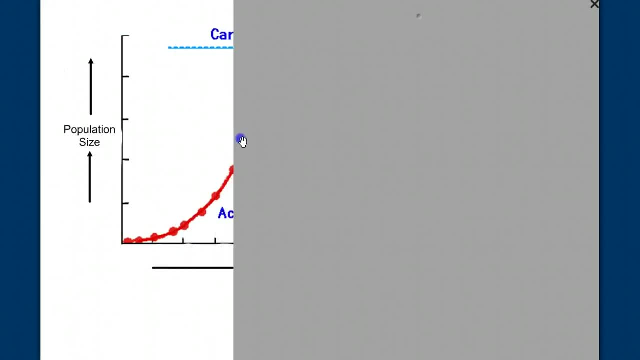 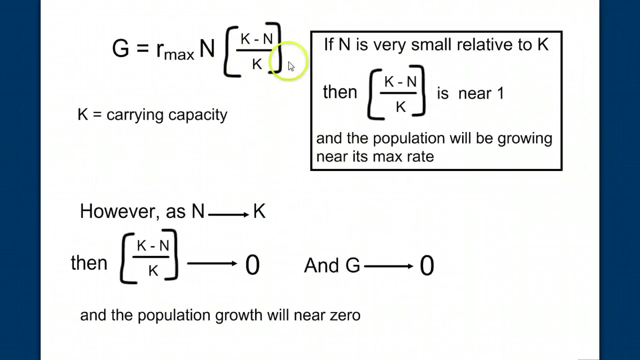 and it'll start to accelerate, creating a graph that we saw before. But at some point, as n- the population size approaches k- the carrying capacity, the rate of growth is going to decrease as this factor nears 0. And eventually it will become 0,.